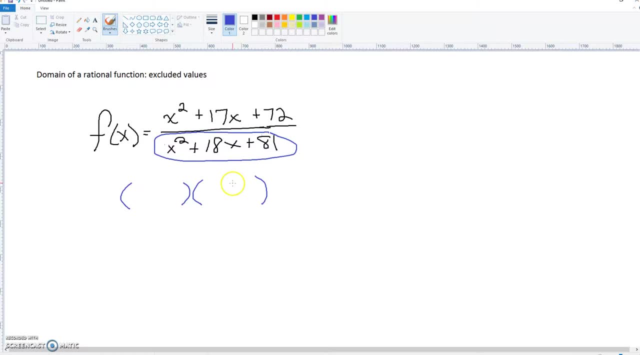 so on. So make sure that you kind of review over your factoring processes. So in this case it's leading coefficient, So we know that both are going to have an x And in this case all of them are plus signs. So that means this is going to be a plus. this is going to be a plus, So that makes 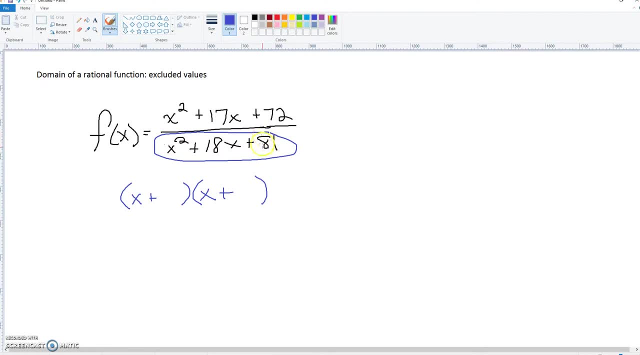 that easy. And now we need factors of 81. That'll add up to get us 18.. In this case it's pretty easy Because we know nine times nine gives us 81. And nine plus nine gets us 18.. So we're gonna put a nine here and a 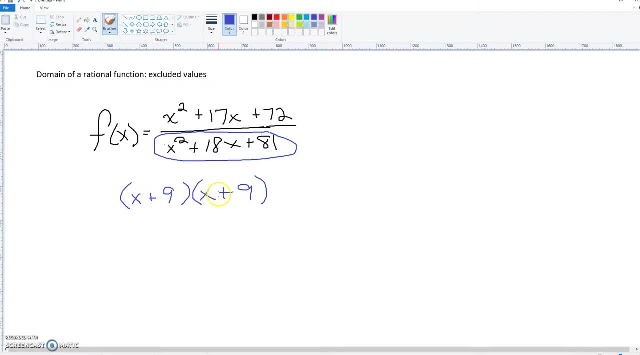 nine here, Okay, and you might not get that every single time in a different set of factors, But once you get to this spot, you're going to go ahead and you're going to separate each of them, So you're going to take your x plus nine. 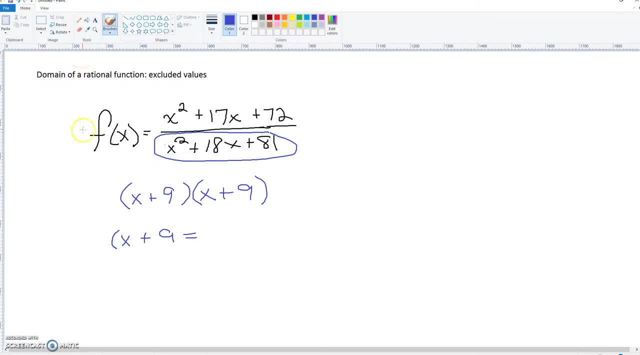 And you're going to kind of set it equal to zero Here. let me kind of erase that. I probably should have put the parentheses there- And you're going to solve for x. So we're going to subtract nine on the side. subtract nine over. 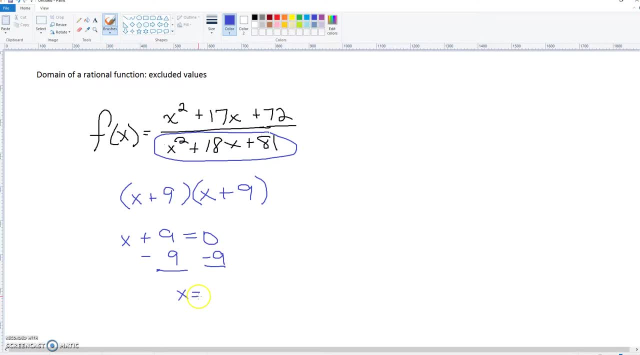 here. So we get x equals negative nine. Okay, if this particular set of parentheses was different, you would do the same thing, And just so you can see, I'll- I'll rewrite it here- Minus nine, minus nine, So we get x equals negative nine. Now we have a double here, So when we go to put the 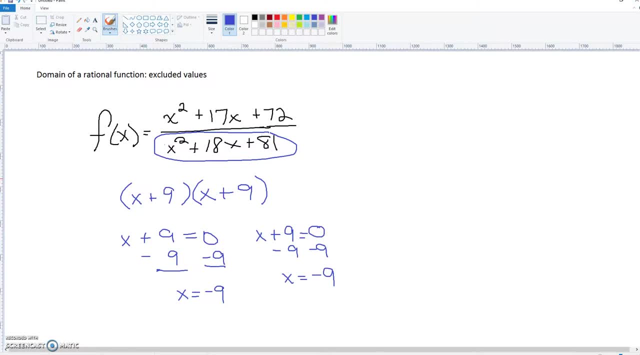 answer into Alex. we only need to put one of the negative nine So we don't have to list negative nine twice. However, if you had more than one answer, you would actually list both. Okay, so in this case we just have x equal- Oh, it's not writing x equals negative nine. Okay, so you would put negative. 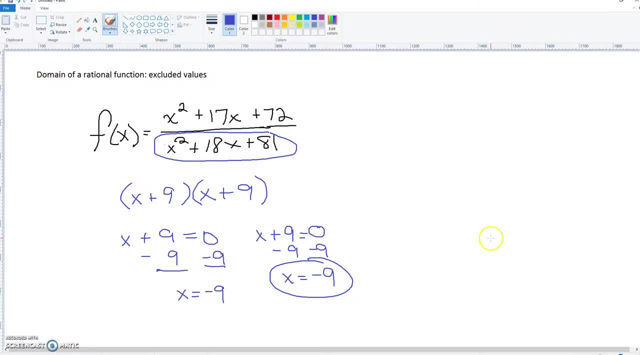 nine into Alex. However, let's say, for instance: let's take this top one, let's pretend that this top one was the denominator of a different problem. okay, and just for humor's sake, I'll kind of scribble something on here, say X plus.